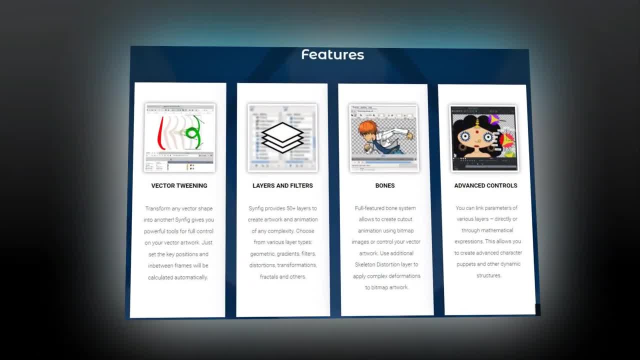 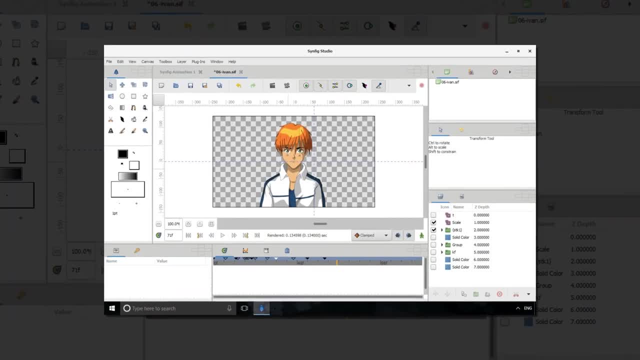 you can use to rig your vector artwork or create cutout animation using bitmap images. It's got a steep learning curve but if you're up to the challenge then Synfig Studio is a great app for beginners and more experienced hobbyists alike. 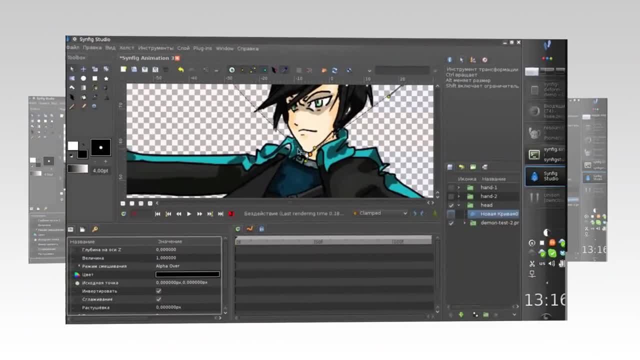 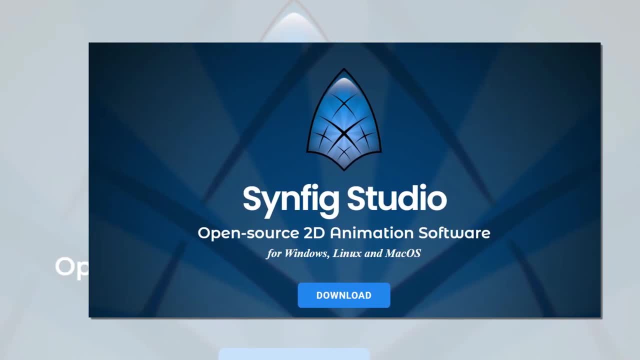 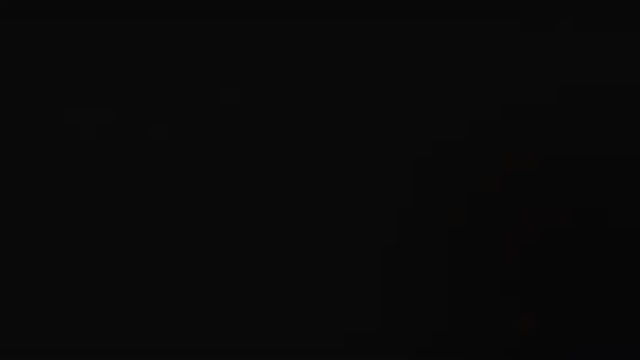 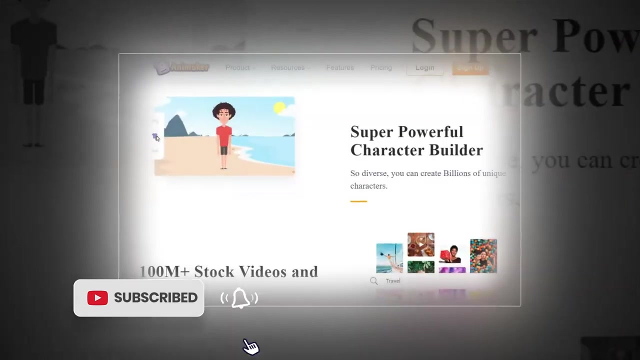 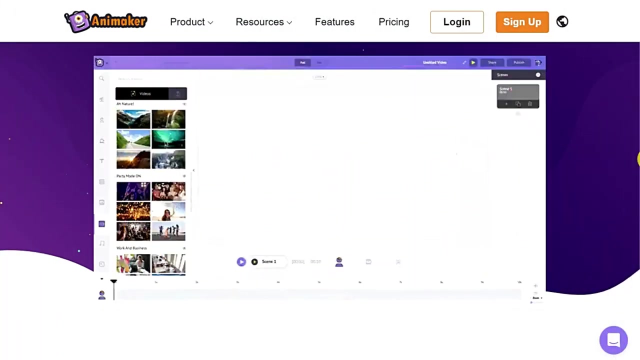 Specifications: Platform: Windows, Mac, Linux, Price: free: Best for beginners and hobbyists: Animaker. Animaker is a cloud-based animated video creation platform that allows users to create and edit animated videos, presentations and infographics. It offers a drag-and-drop interface, a library of templates and assets and a wide range. 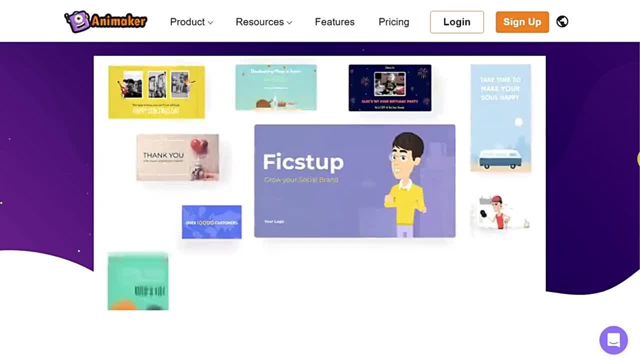 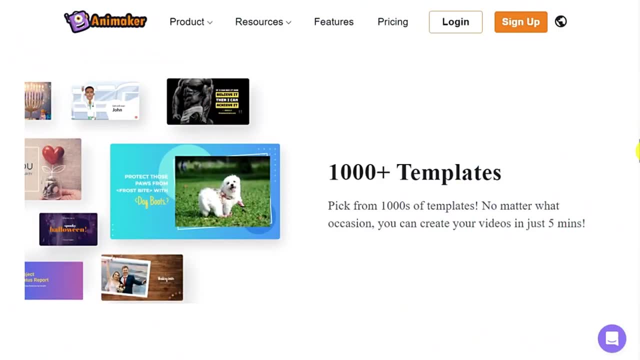 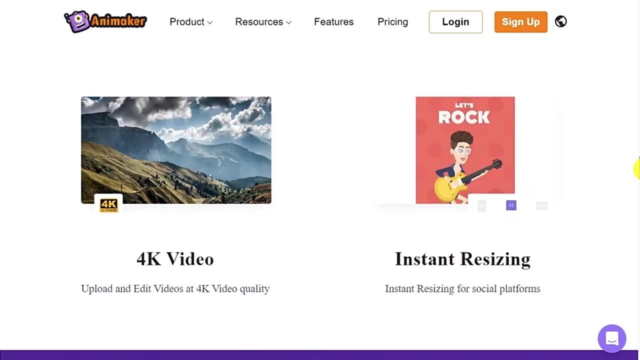 of features, including text-to-speech music and sound effects. The software is completely web-based- you don't have to install anything- and very easy to get started with, With full HD support, horizontal and vertical video layouts and pre-made graphics. you. 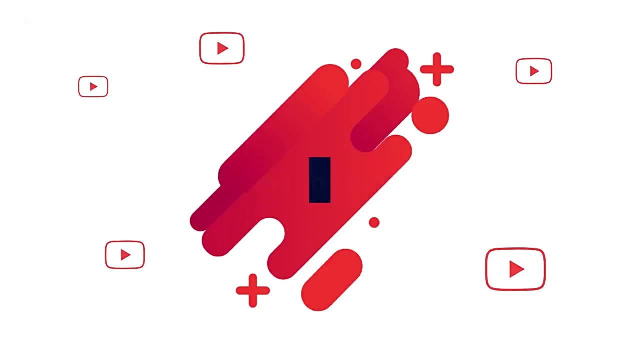 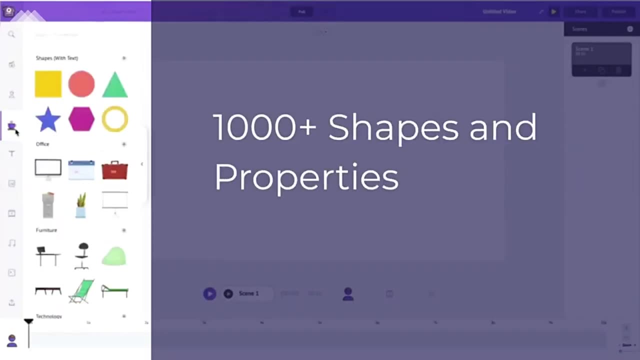 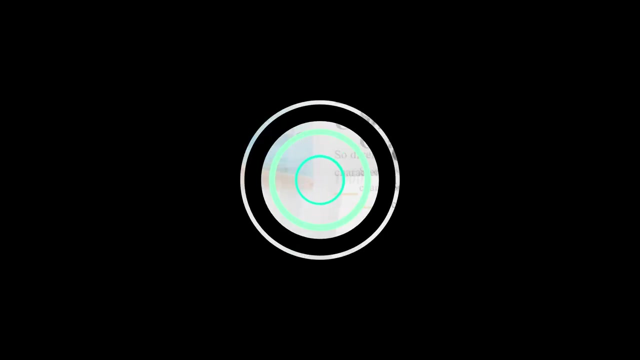 can create fun animated videos in no time. Audio features include text-to-speech, the option to add background music and sound effects, and voiceover. You can choose from Animaker's library of sounds or upload your audio. Animaker offers a variety of templates. 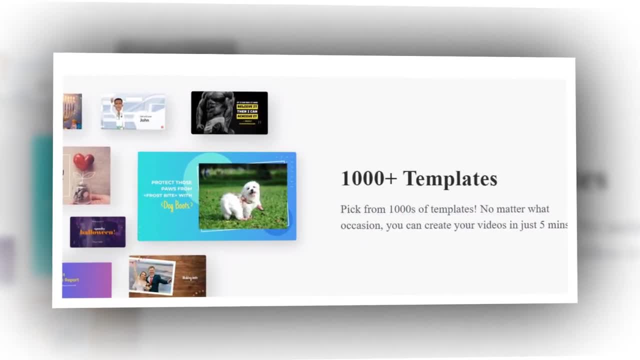 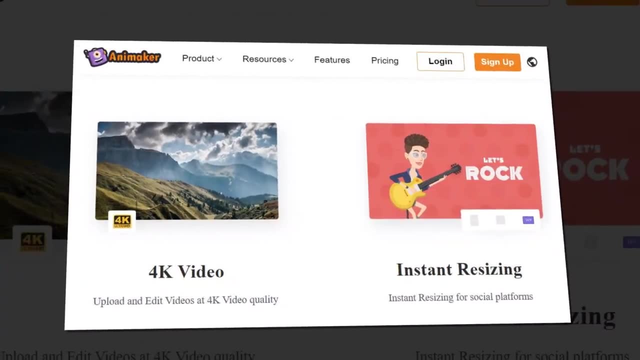 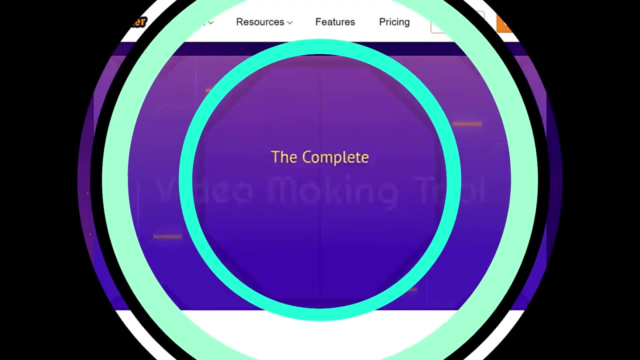 The templates are customizable, with the option to add text, images, music and sound effects. They are designed to be user-friendly and provide a starting point for creating animated content. Overall, Animaker is a useful tool for creating animated content, and its features and templates. 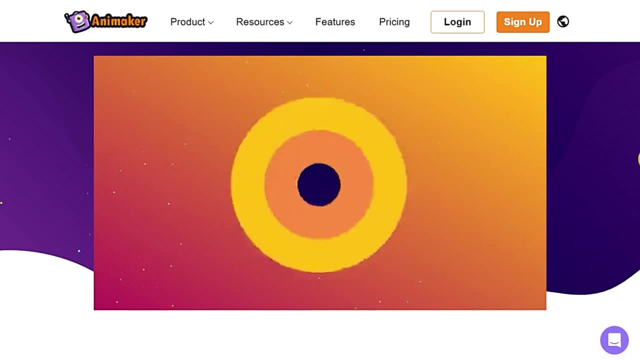 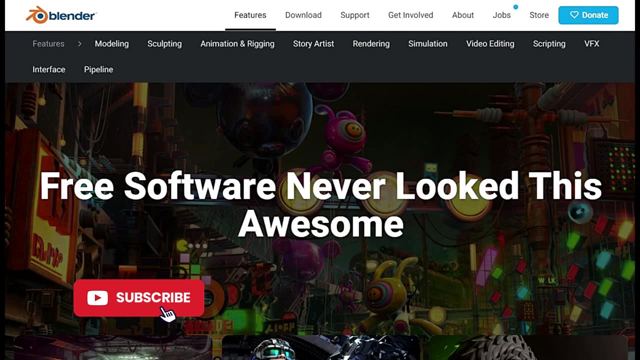 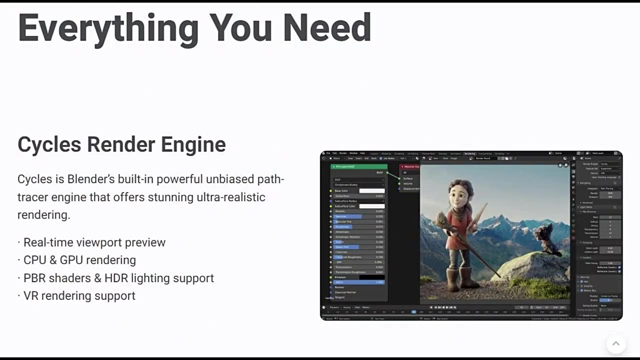 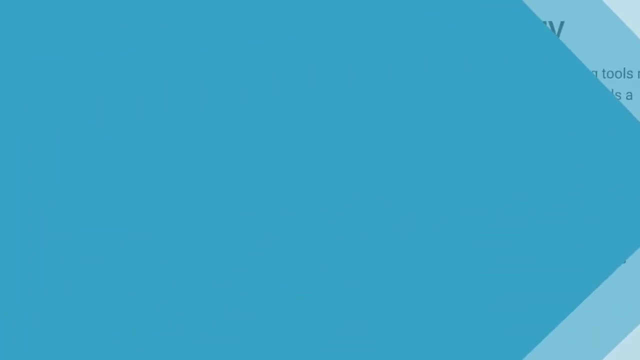 make it a good choice for those looking to create professional-looking videos. Blender is a powerful open-source 3D creation software used for making animations, models, artwork and more. It offers a wide range of features, including modeling, texturing, rigging, animation and. 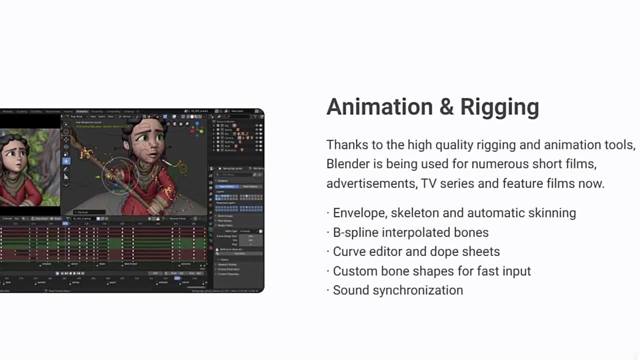 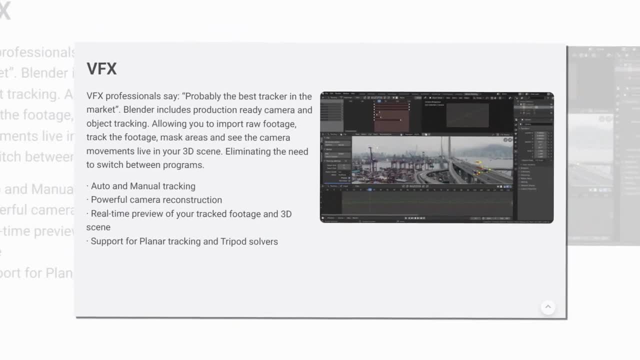 simulation. Blender has a large user community and a vast online library of tutorials and resources, making it accessible for artists, video editors and video editors alike. It's also available on all types of video games. Many professionals in the film and game industries use Blender for their projects. 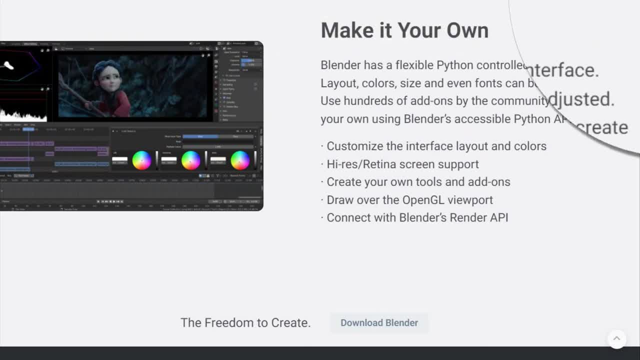 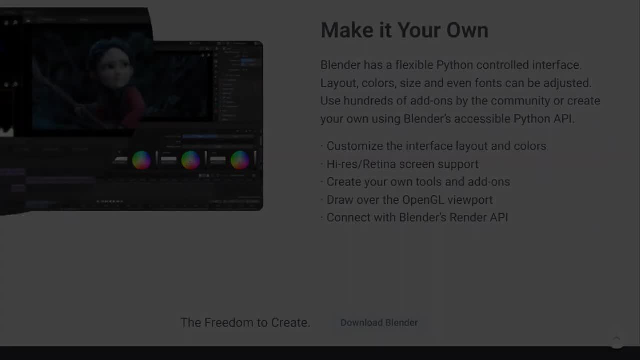 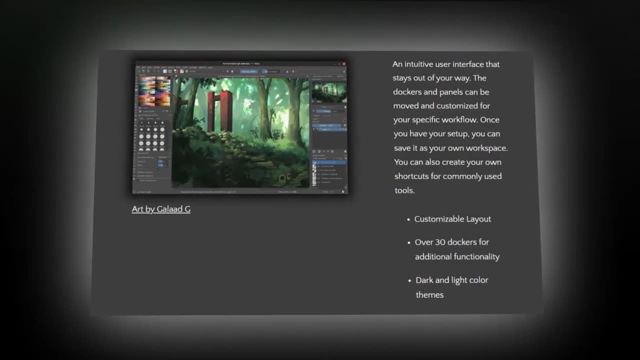 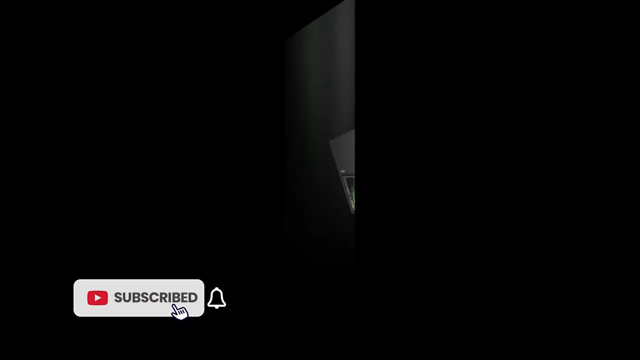 Overall Blender is a versatile, free alternative to paid 3D software and has a strong reputation in the 3D creation industry. Krita is probably one of the most highly regarded free animation applications. ideal for hand-drawn animations, Krita includes over 100 pre-loaded brushes, each with various effects. 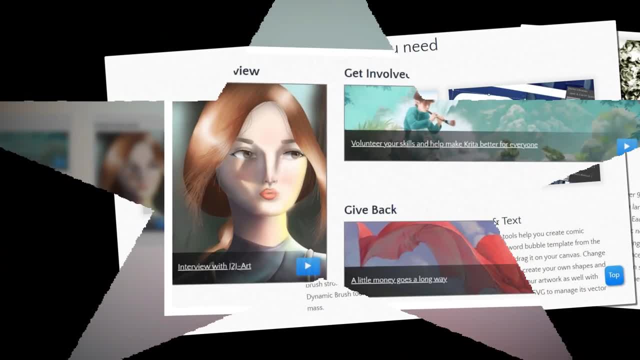 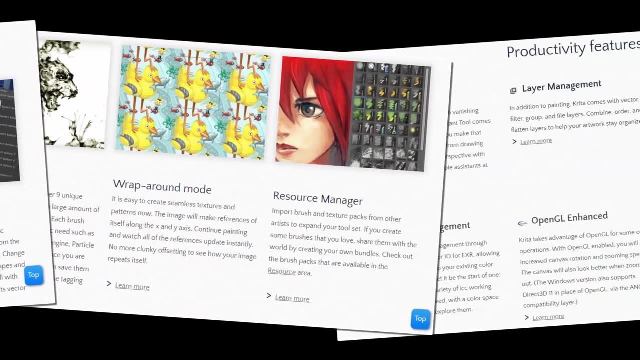 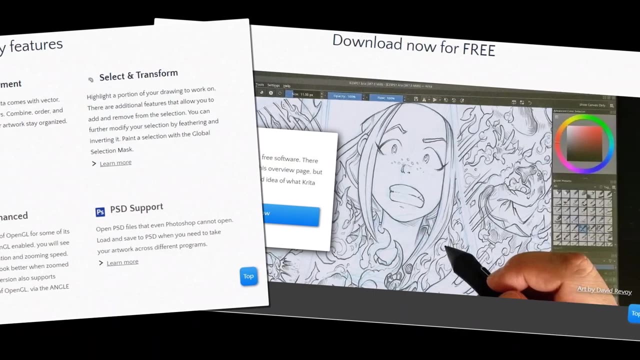 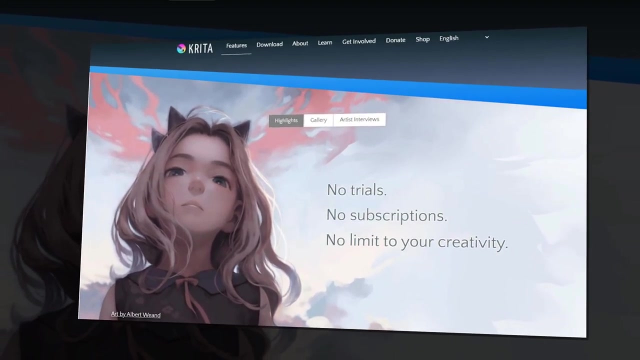 Users appreciate Krita's intuitive user interface, customizable workspace and the ability to create high-quality digital paintings and illustrations. It supports a variety of file formats, including PSD, and offers a robust set of tools for creating animations and graphics. Overall, Krita is a great choice for beginners or hobbyists. 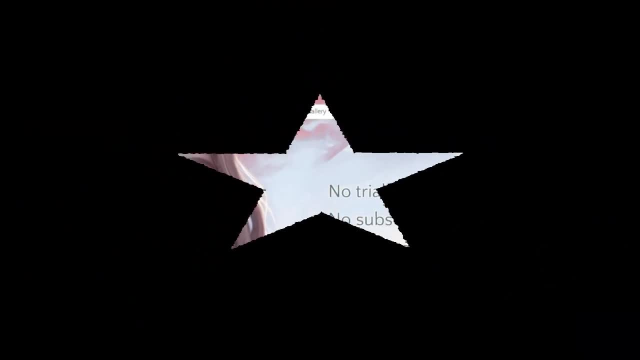 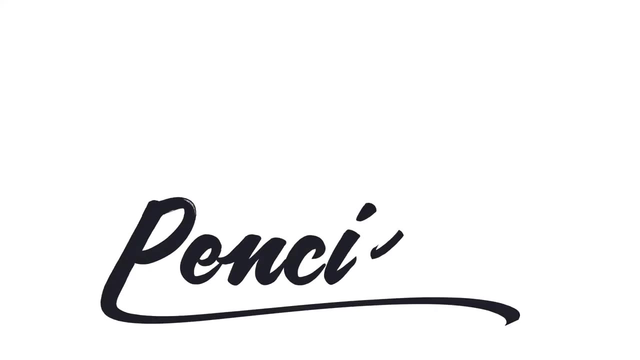 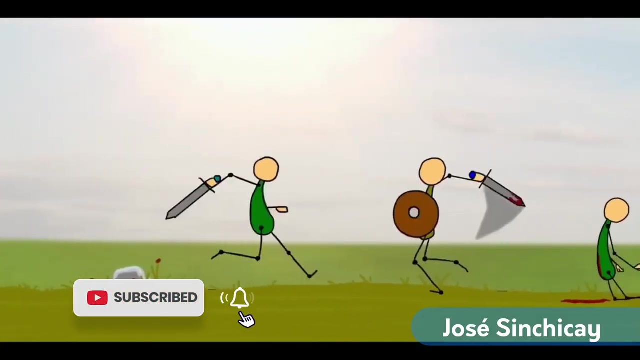 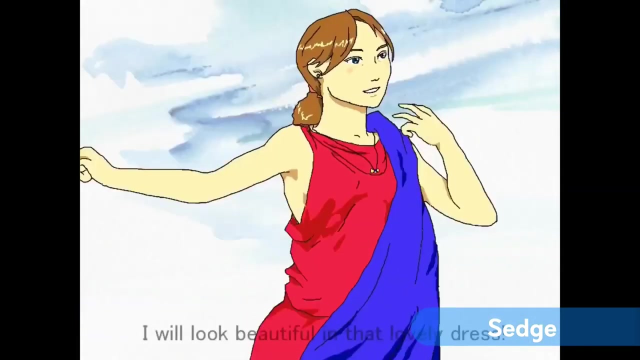 looking for a free and open-source digital painting software. If you're looking for a lightweight animation solution that's not only open-source and free but also easy to learn, then Pencil 2D Animation is an excellent place to start. You can use it just for fun or create videos to promote your product. 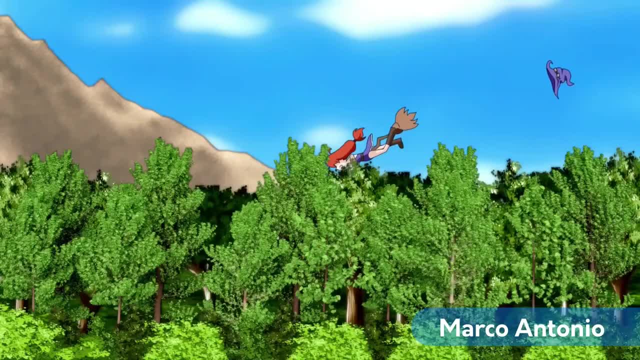 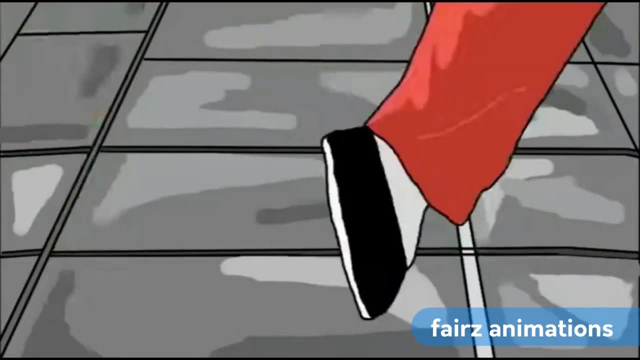 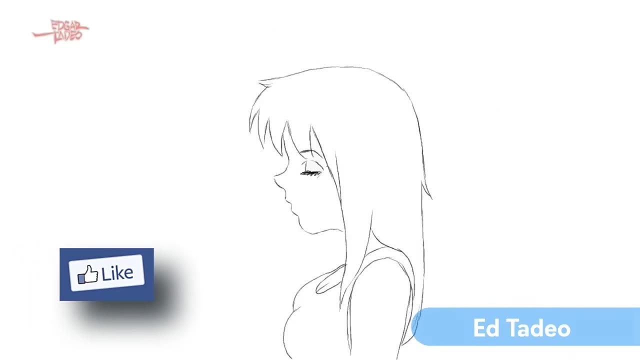 The interface is simple and easy to use. Plus, there are tons of tutorials on Pencil 2D's website to help get you started. Other Features: Image and Audio Import. Switch between raster and vector workflows so you can sketch, ink and paint. 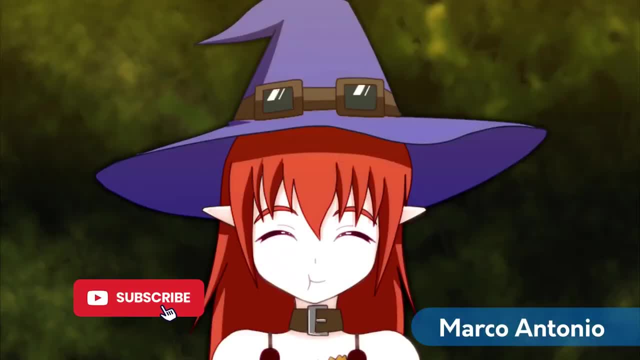 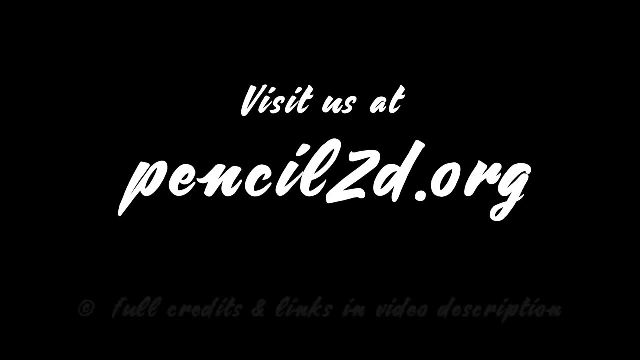 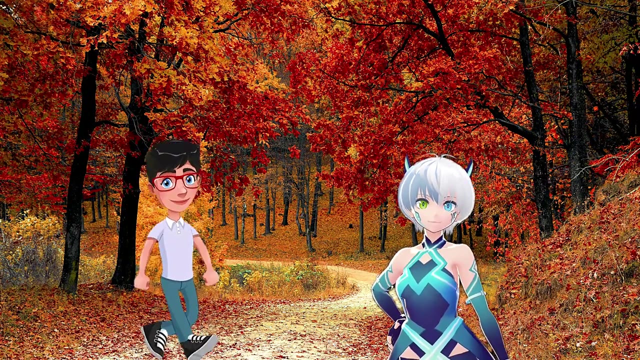 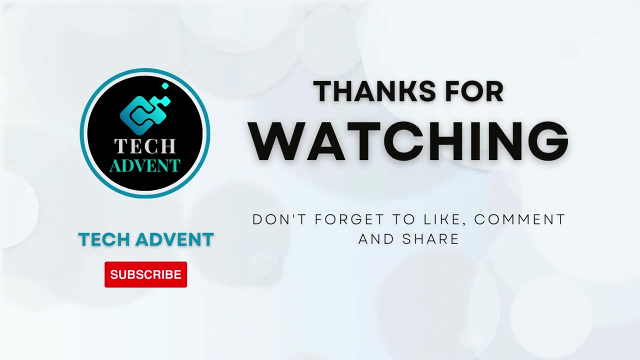 Adjust Frame Rate, Add Distortion and Lighting Effects, Toolbar Customizations, Pressure Sensitivity, Multiple Export Formats. These software provide a user-freindy interface and a variety of tools to help beginners create animations easily. Please check out communities you may see in this section For details. keep checking the sheet and to supportיתhroughqato. Let's start writing pictures, Or perhaps the best toolwe band of race in life to write music. Photoshop, Yes, Photoshop, Hello.